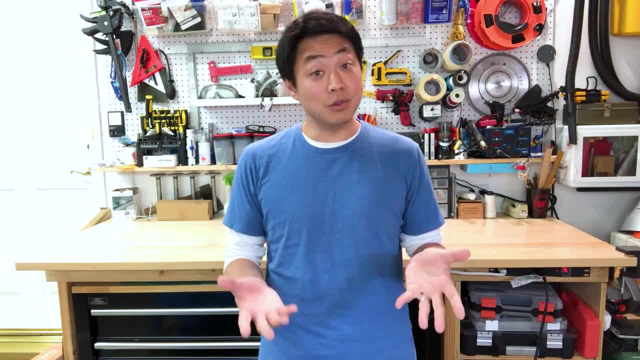 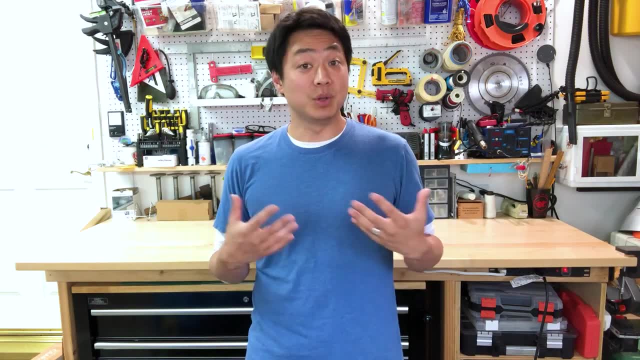 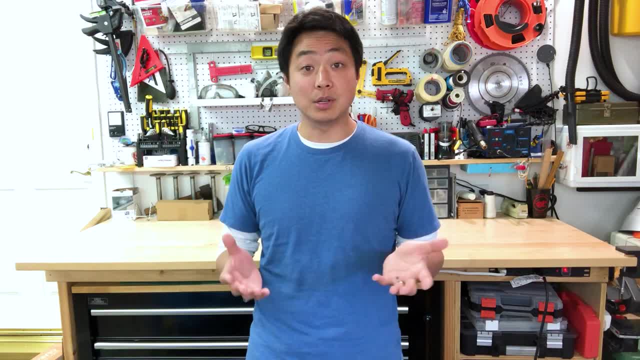 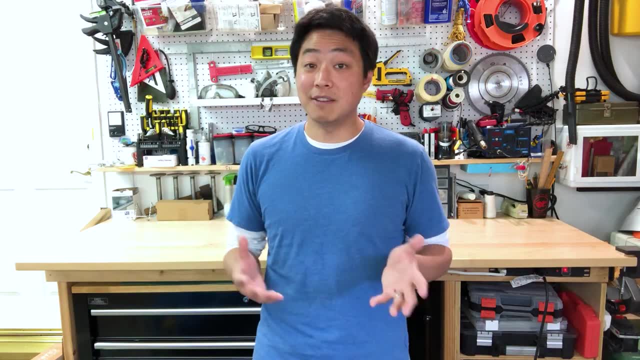 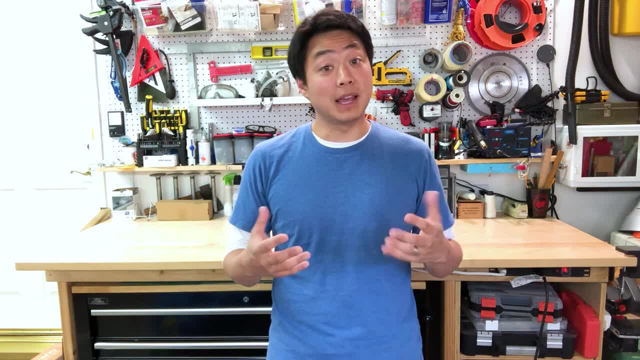 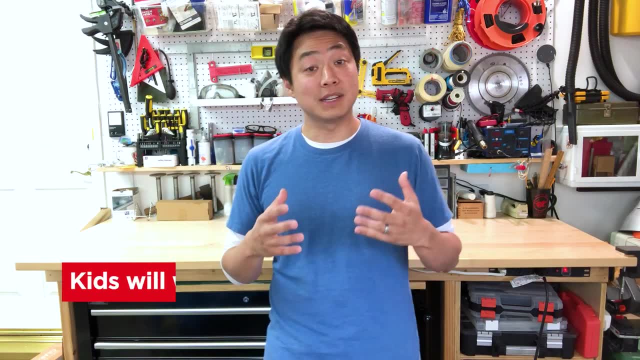 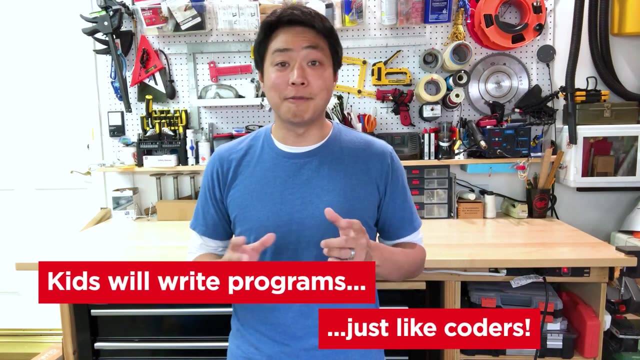 to go with their robots every step of the way, so they give a preset list of directions that they call a program. Now, today's activity is going to give kids an opportunity to be exposed to this concept, as well as a fun way to practice thinking things through before they act. Pretty valuable. 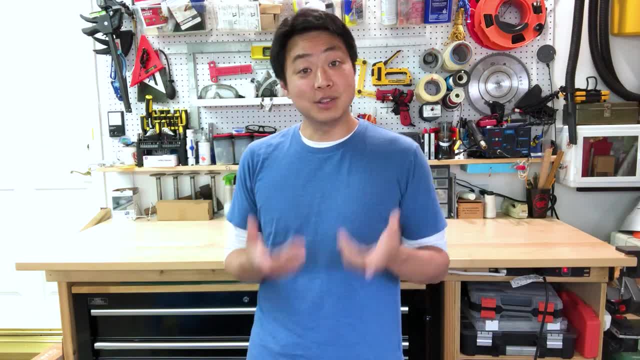 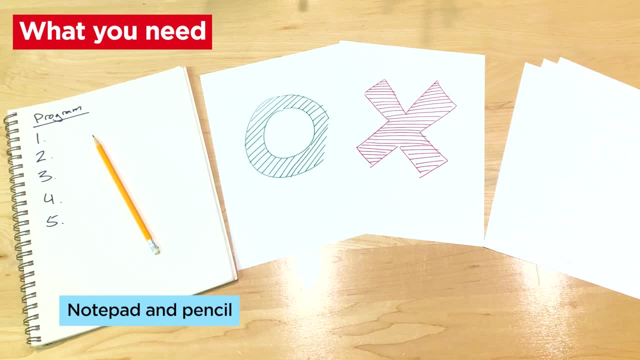 for coding as well as life in general. But to do this activity, here's what you're going to need. Kids are going to need a notepad and pencil to write down their programs. They'll also need something to mark a starting and stopping point. Now, this can be as simple as 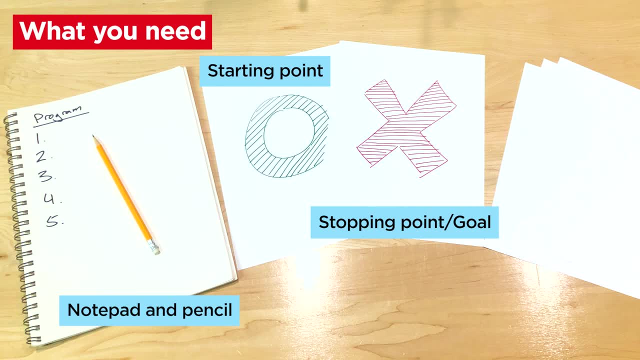 something drawn on a piece of paper like a star or a green circle for the start, or an X or red circle for the goal. Lastly, you'll need to lay out a large grid that kids can walk on. You can make your grid from things like paper chalk or cheap paper plates or even playing cards, but whatever you, 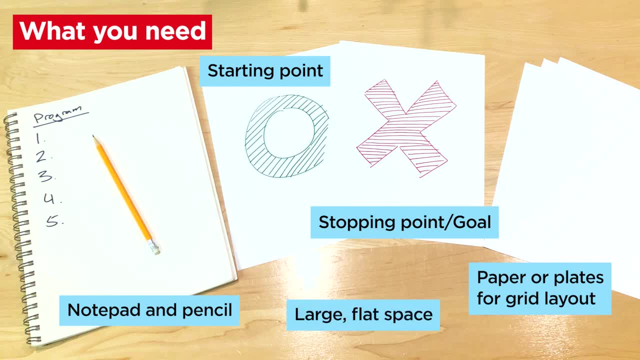 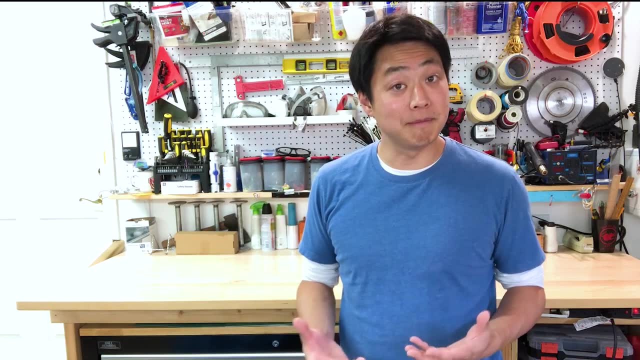 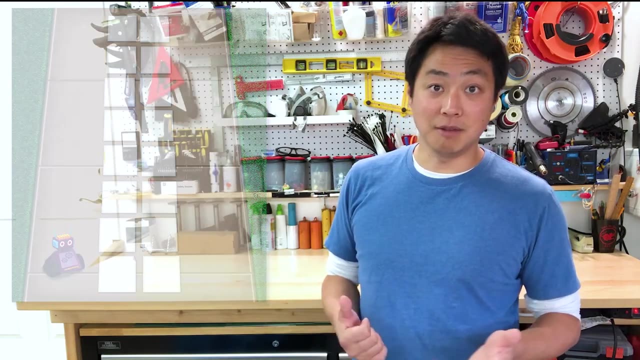 use, know that it'll probably get messed up. You'll also need a large flat space to lay out the grid. Once you have your materials, let's set up the grid depending on however many units you have. For example, if you have 16 units or 16 pieces of paper, you can set up a 2x8 grid, a 4x4 grid. 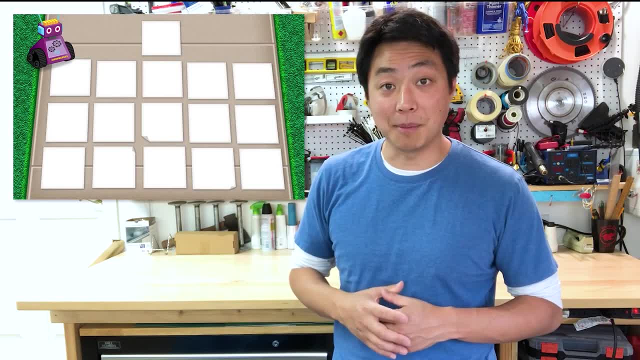 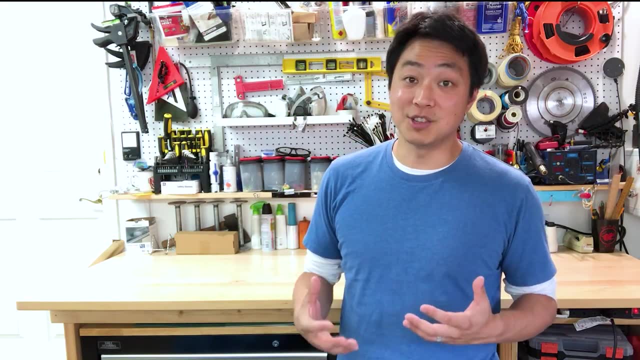 or even a 3x5 grid with that last piece of paper at the top. I'll tell you right now, though: the more units you have, creating a larger grid will make the kids programs a lot more fun and interesting. Also, make sure that your units are spaced about one child size. step apart, Kids are going to be. 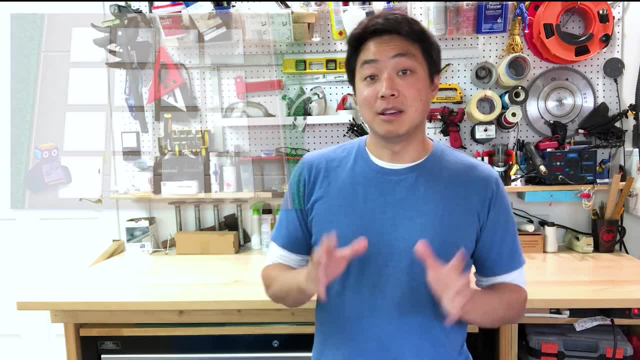 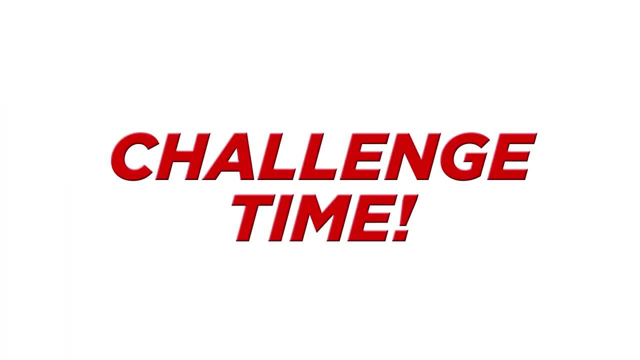 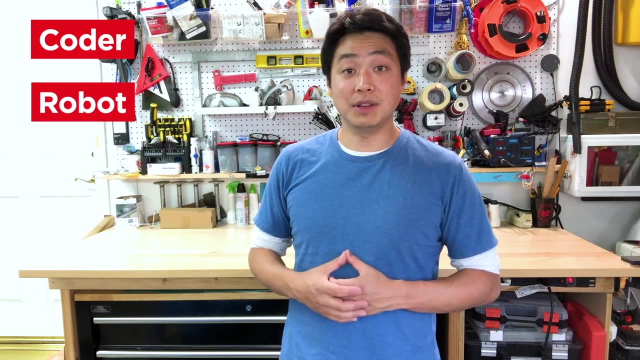 walking from unit to unit, so you don't want them to be too far. Once you have your grid set up, let's get started. This activity really requires two players. You need a coder and you need a robot. Now, you can do this activity with one kid, but encourage them to find or even make a robot that. 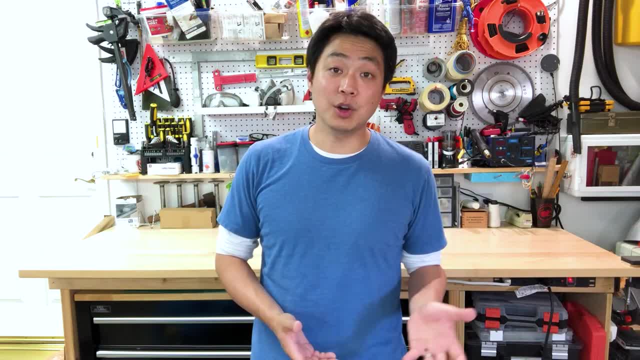 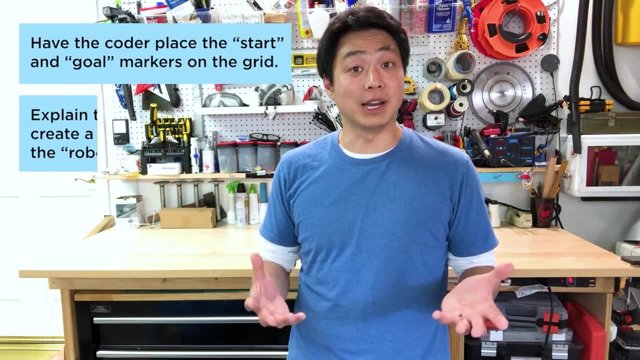 they can use to help play that part. Either way, have the coder play the grid and, if you're not sure, place the start and goal markers somewhere on the grid and explain to them that the challenge of this activity is to create a program or a list of directions that will help guide the robot from. 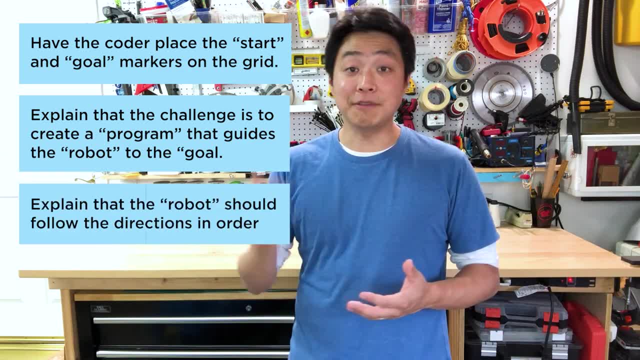 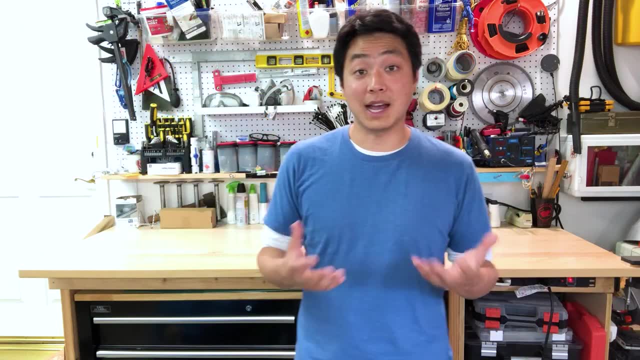 the start to the goal. Explain to the robot that they have to follow the directions in order and that they can only walk forward in the direction that they're facing. So if the first line in the program is the number three, that tells the robot that they should walk forward three units. 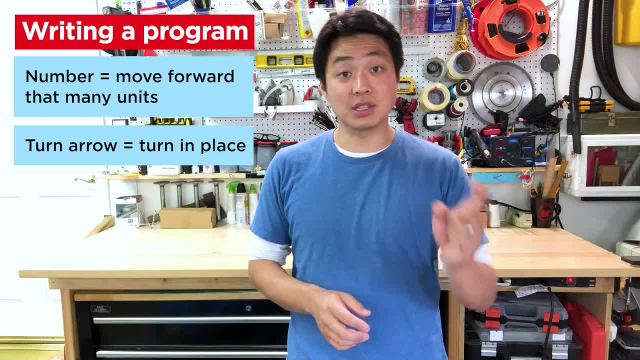 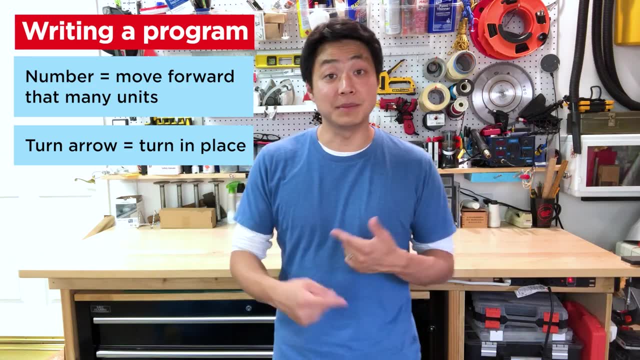 So if the next line in the program says turn right, or it shows a little arrow that tells the robot to turn in place, stop and then move to the next line in the program. Do this until they've come to the end, at which time look around and see where they ended up. 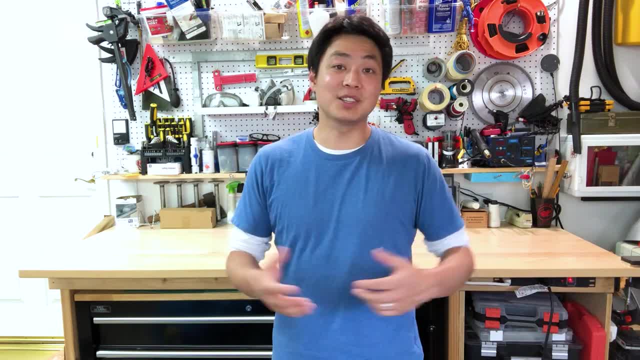 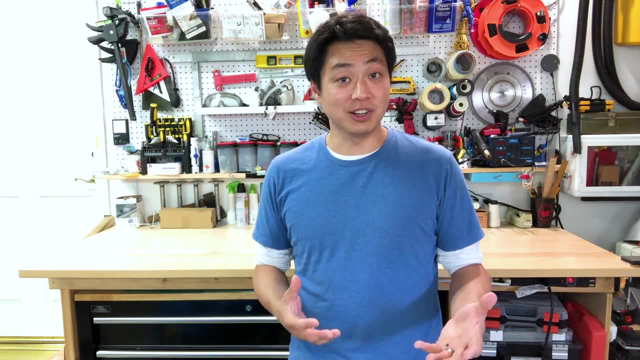 Is the robot standing on top of the goal marker? If so, great, That means the coder wrote a totally successful program and that the robot will find its way to the goal every single time. If the robot is not standing on the goal marker, have the coder look back through their program. 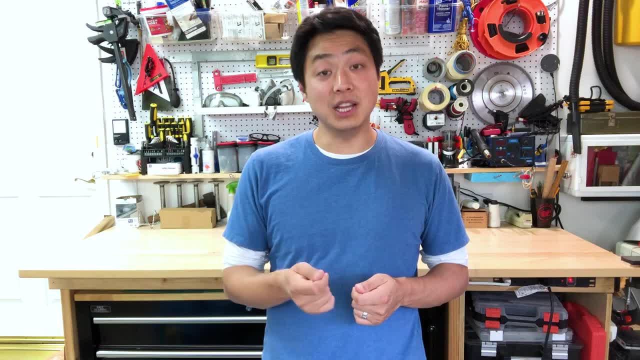 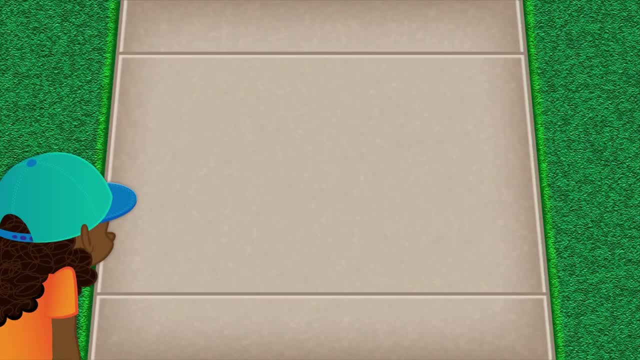 and see where they might have misled the robot. Have them make the change and then try the program again. Now here's a little program that I've wrote. Let's run through this one together. My program is for a 4x4 grid with a start and. 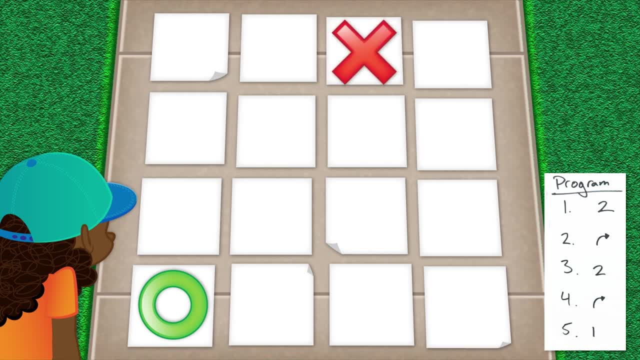 stop markers placed here and here. Once the robot is at the start marker, we're ready to go. The first line in the program is a two, so the robot will move forward two units. The next line shows a right arrow, so the robot should turn in place. The next line is a two. 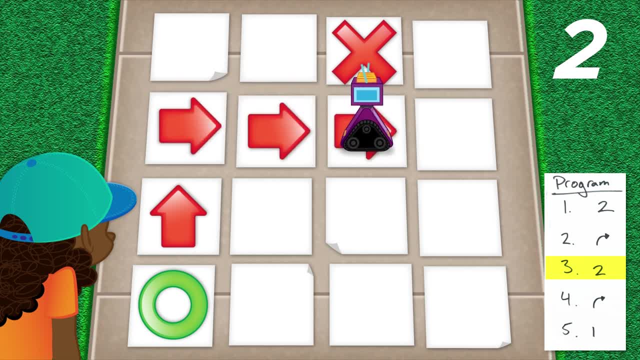 so the robot should move forward two more units. Next is another right turn, so the robot will turn in place again. Finally, the last line is one. so the robot moves forward one unit. Okay, so the program is over, and the robot clearly didn't make it to the goal like we. 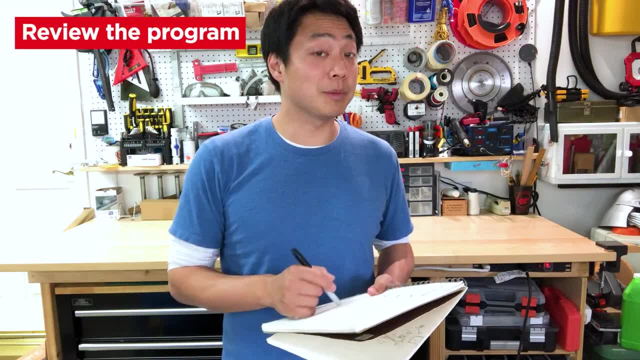 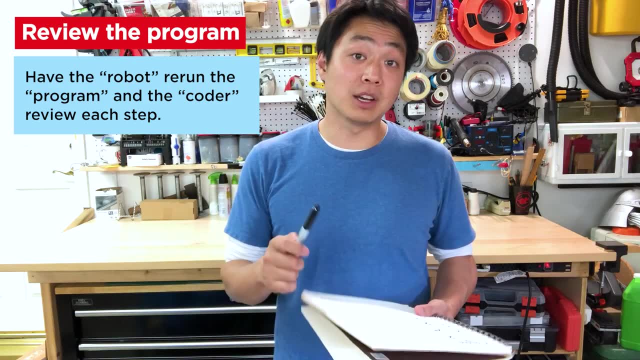 had originally hoped. Now, at this point, the coder should be reviewing their program, trying to see what exactly went wrong. A good way to do this would be to have the robot rerun the program, having the coder follow along at each step Once they find out a place that they